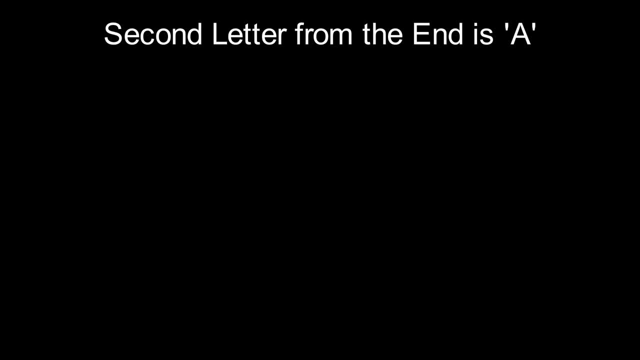 strings that accepts a string. if, and only if, the second to last letter is a, We'll have a set of states: q0 through q4.. The symbols will be a, b and the edge markers. q0 is a start state. 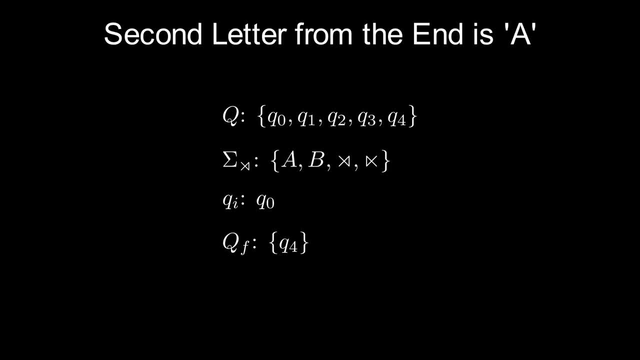 and q4 is the final state. I'll list the transitions as we traverse through the string. We'll use the example string b a a a b. Since we're using edge markers, we need to add them to the string before giving it to the automaton. 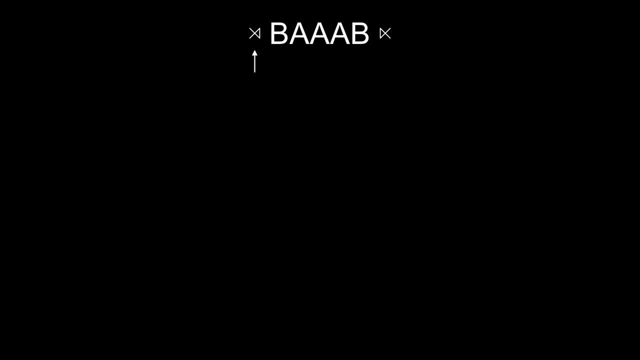 We're starting from the left marker instead of the first letter. What we're going to do is read until the end and then look two characters backwards. So when we read this left edge marker, we're going to transition to the same state and explicitly mark that. 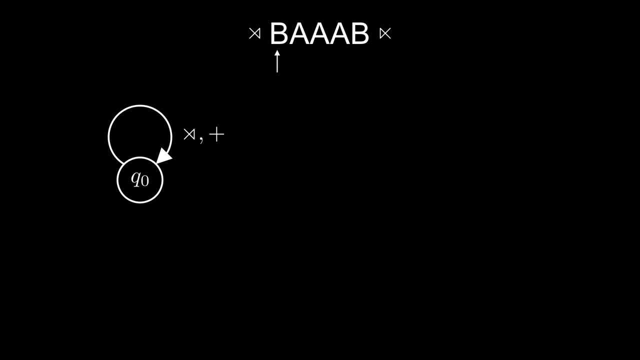 we're moving forward in the string. When we read an a or b in this state, we're going to do the same thing. This is because we don't care about the symbols until we start counting back from the end. So we keep transitioning to state q0 until we read the right edge marker When we do. 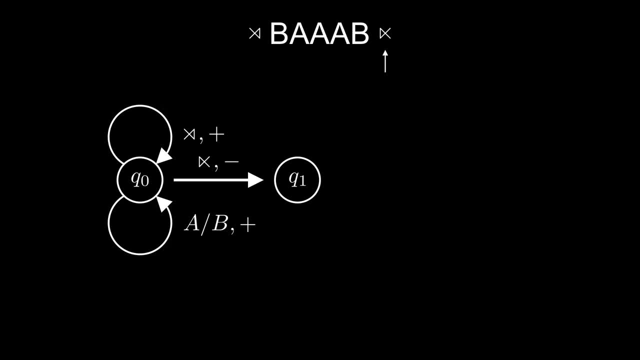 we're going to transition to a new state. This transition also indicates that we're going to go backwards, So the next character we're reading is the last b From here. finishing the automaton is just like checking if the second letter is a in a one-way automaton, but with the indication: 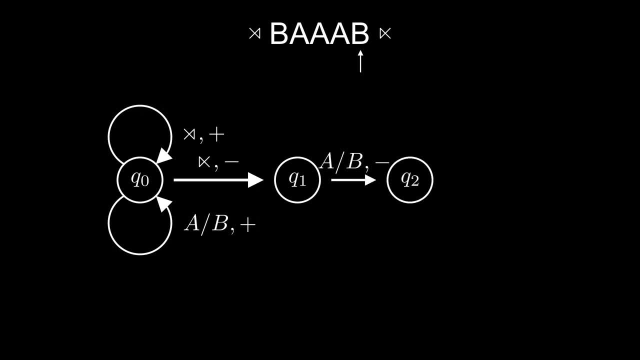 of backwards movement. We transition to another state regardless of the letter. Then we transition to the accepting state if the next letter, which is the second from the end, is a, or to another non-accepting state if it's b. That's it. Now this automaton actually has one more state than the. 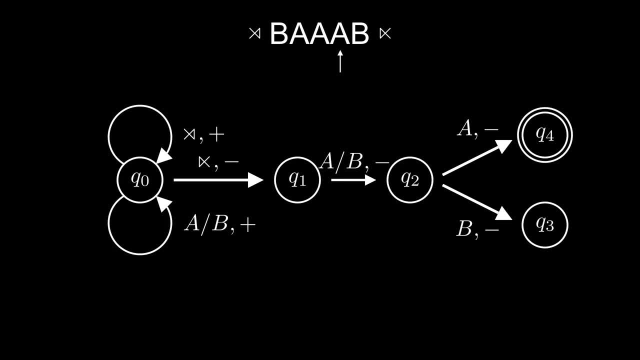 smallest excepting state. This automaton actually has one more state than the smallest excepting state. But if we want to go further back- third, fourth, fifth letter- from the end- then for each additional letter we add one more counting state after q1.. Going back further in a one-way automaton: 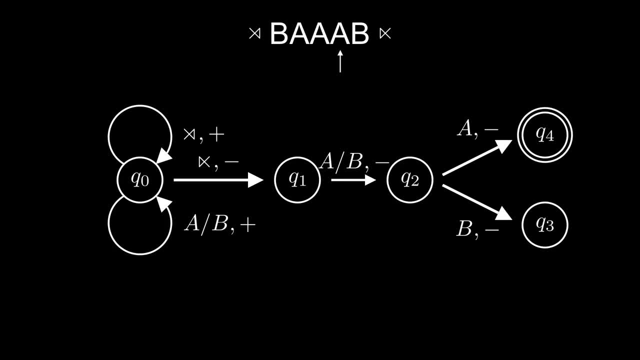 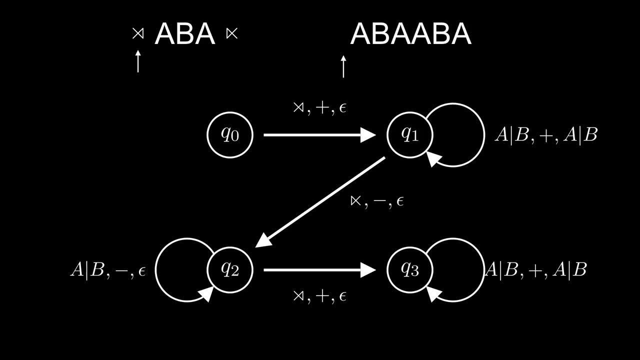 requires an exponentially larger number of states. So, even though they're equivalent in computational power, two-way automata can make things a lot simpler. Two-way transducers are more powerful as they're able to perform certain operations of arbitrary length like copying and